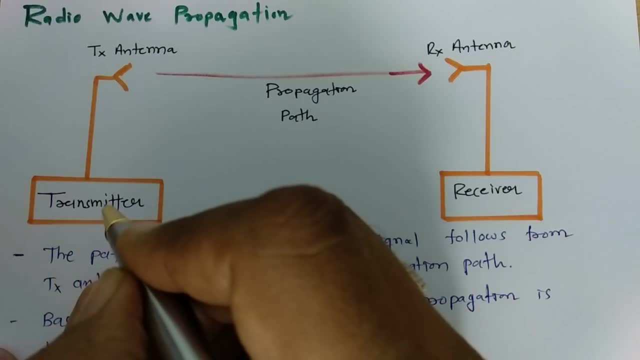 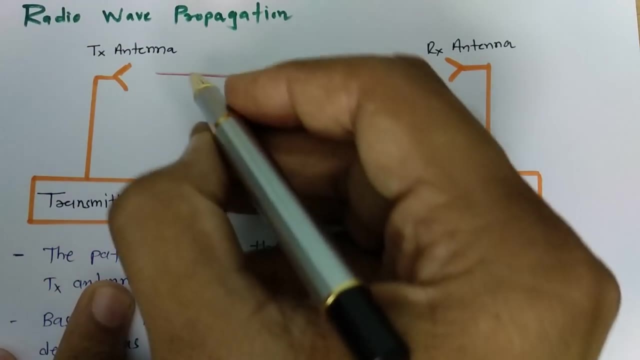 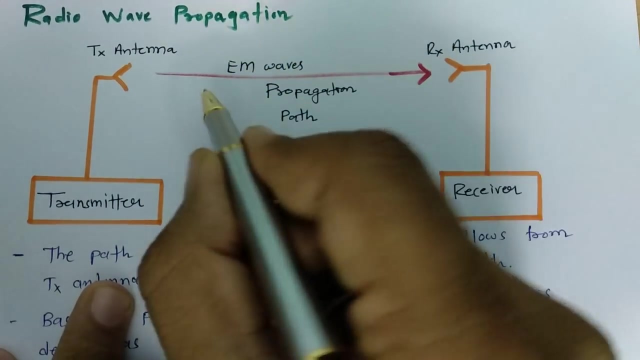 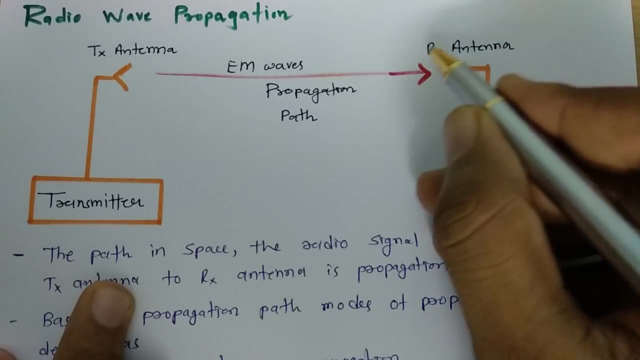 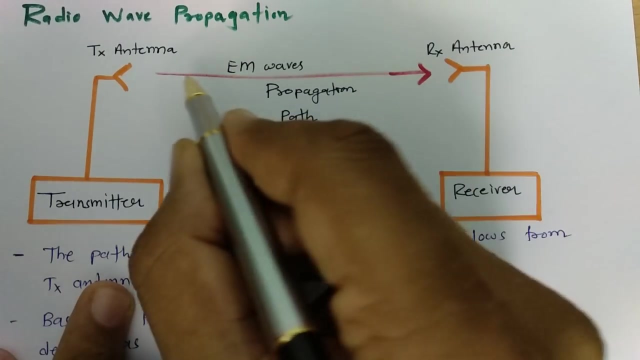 we have a transmitting circuit which is giving transmitting signal to transmitting antenna and then transmitting antenna that will radiate electromagnetic waves. So it radiates EM waves and these EM waves that is propagating along propagation path and then it is getting received by receiving antenna and that signal is given to receiver. So basically, when it propagates, 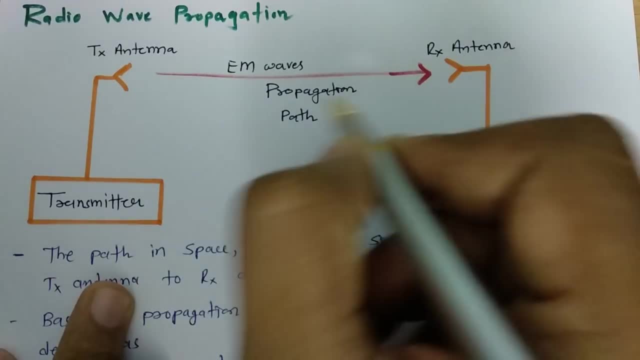 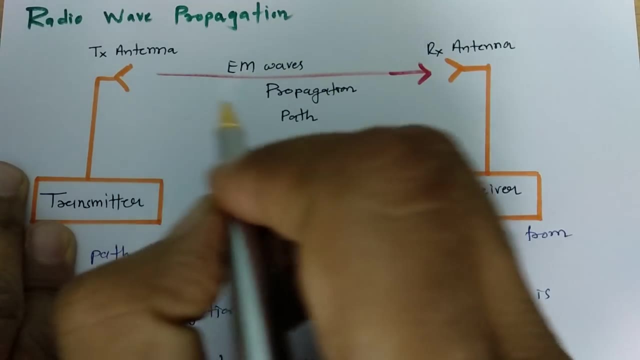 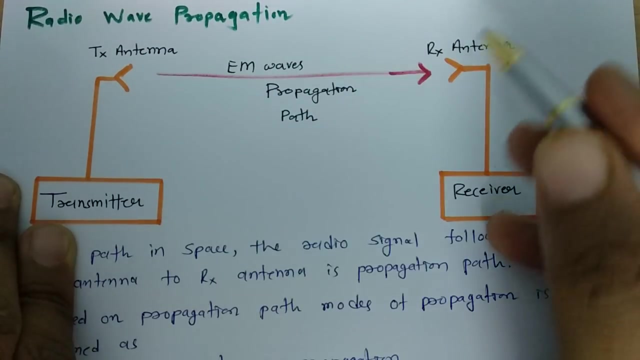 in a channel, the way it propagates based on that. that is what propagation mode. So in this session I'll be explaining different types of propagation which is happening, of radio wave propagation from transmitting circuit to receiving circuit. So let us begin the session with basics of those things. So first, 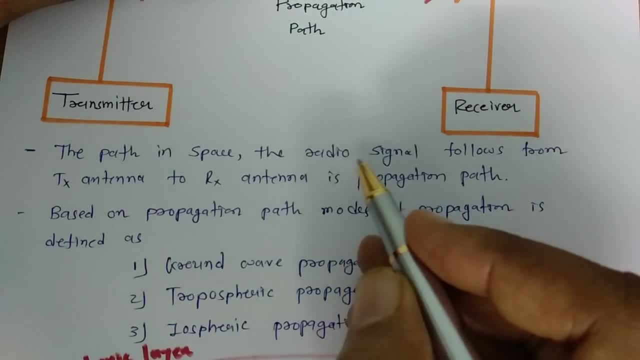 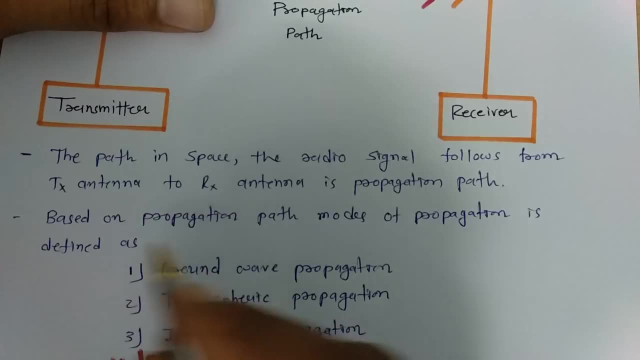 is the path in space the radio signal follows from transmitting antenna to receiving antenna. that is propagation path And, based on propagation path, modes of propagation, is defined as ground wave propagation, tropospheric propagation and ionospheric propagation. So, based on propagation path, modes of propagation of radio wave, that has been defined in three categories: ground wave propagation, tropospheric propagation and ionospheric propagation. 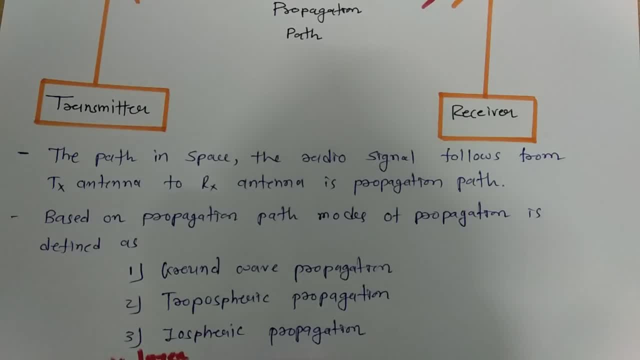 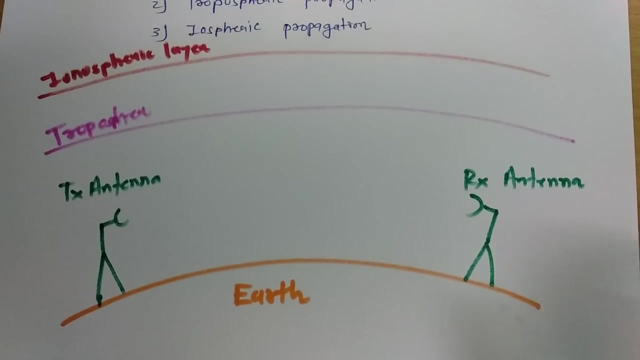 So in today's session I will be explaining little bit basics regarding all three propagation and detailed explanation that I will be going to explain in next few sessions. So when you see earth, so by this orange color I have shown this is earth surface and we have transmitting antenna and we have receiving antenna. 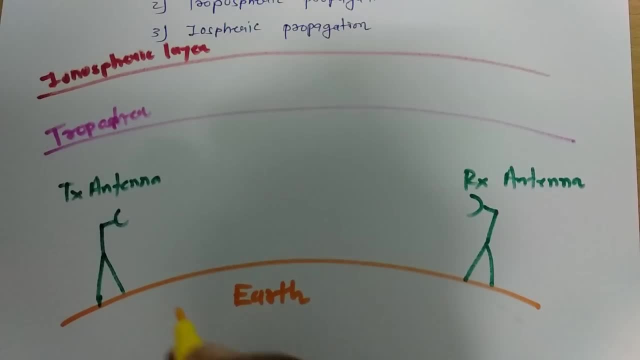 Now for ground wave propagation. Electromagnetic waves, that is propagating along the ground. So when we send signal that is getting propagated along the ground to receiving antenna, So in ground wave propagation transmitted signal will get received at receiving antenna along the ground. 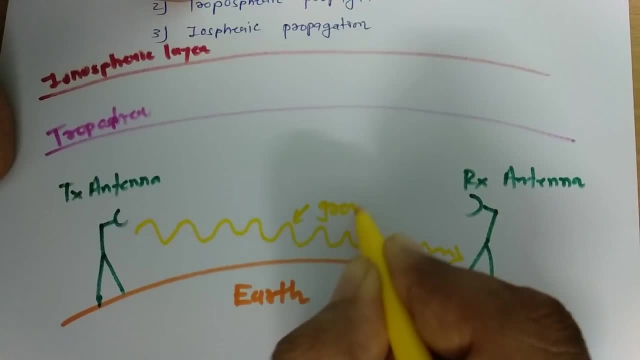 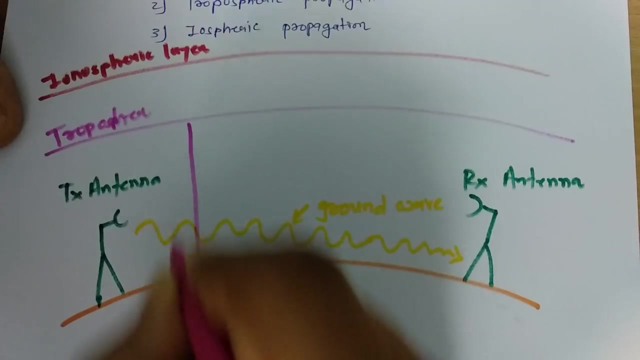 So this is what ground Wave propagation, in which signal from transmitting antenna will get received to receiving antenna along the ground. So this is about ground wave propagation. Now, when we talk about tropospheric propagation, then above earth surface by a distance of 16 kilometer. 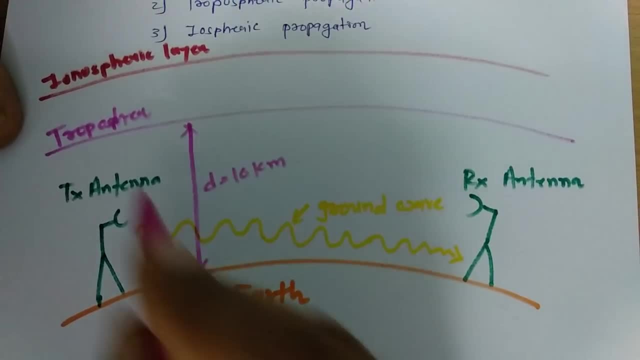 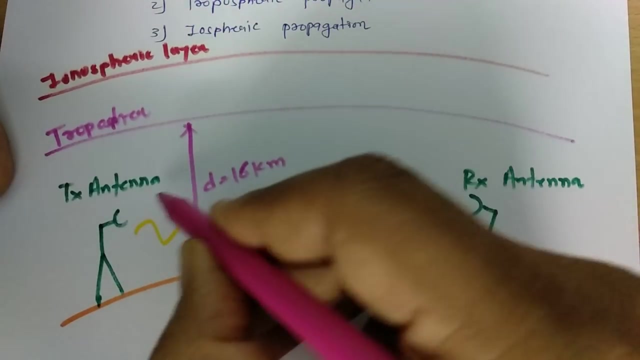 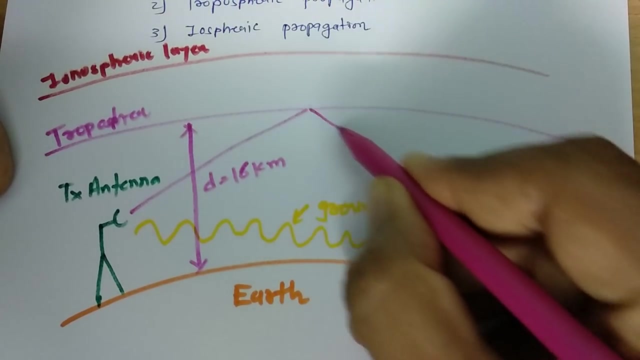 There is tropospheric layer At the distance of 16 kilometer. there is tropospheric layer. Now, when we send signal by transmitting antenna on tropospheric layer And then, after scattering or reflection, it will come back on the earth surface and it is getting received by receiving antenna. 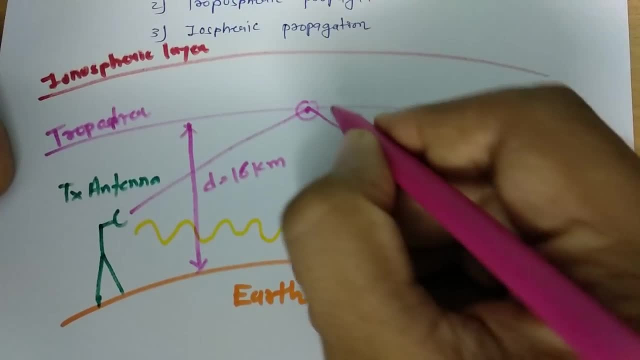 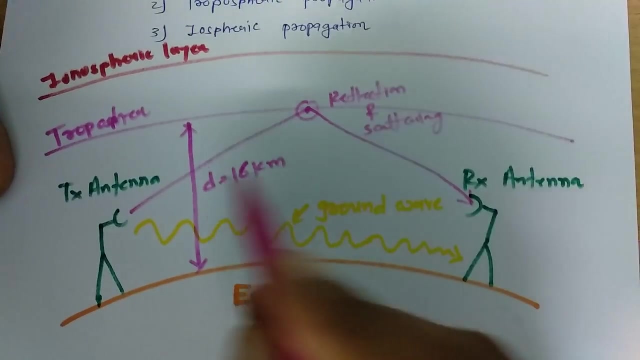 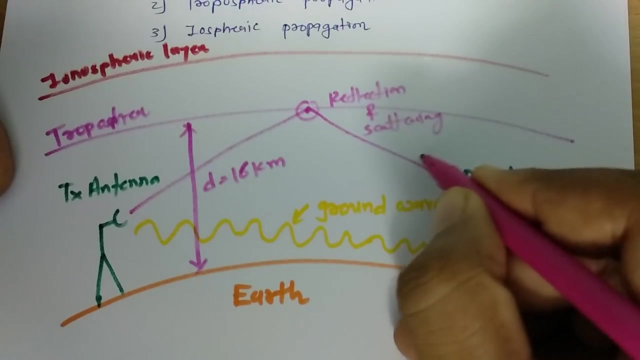 So here there are two things which is happening: Reflection as well as scattering, And that happens from tropospheric layer, which is about above 16 km from the ground. So when this wave is getting reflected back to this receiving antenna, this wave propagation that is called as tropospheric propagation. So this is a case which is there, with tropospheric propagation. 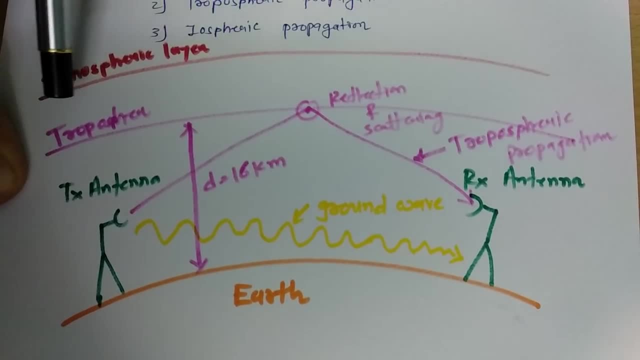 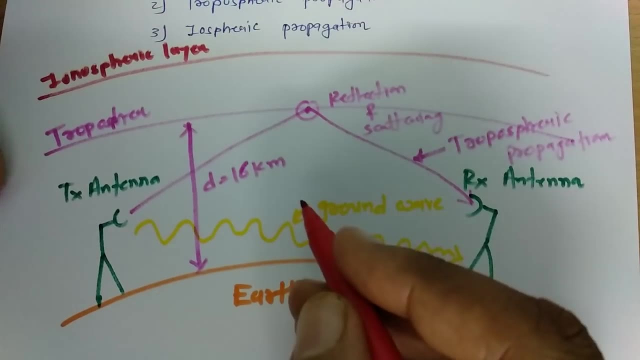 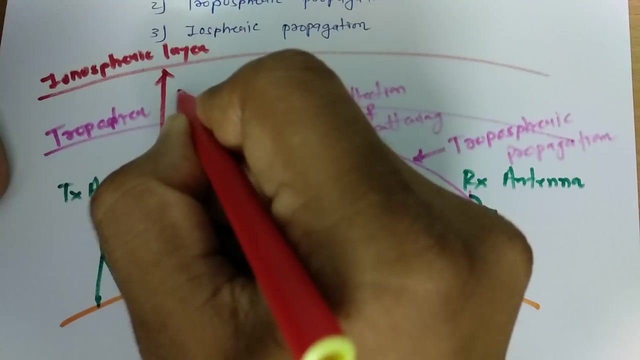 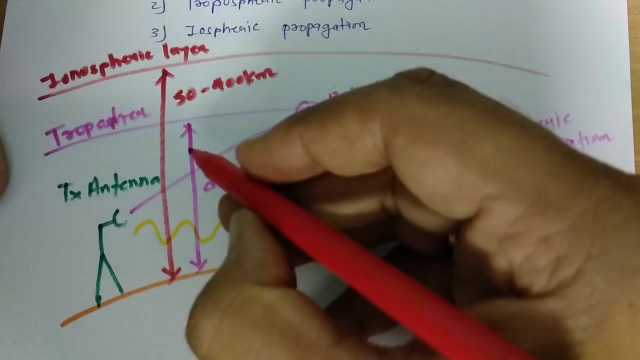 Now I will explain third category, which is ionospheric propagation. Now, when we talk about ionospheric layer, so ionospheric layer that is above from earth's surface by 50 to 400 km. So what happens is when we send signal from transmitting antenna to ionospheric layer. 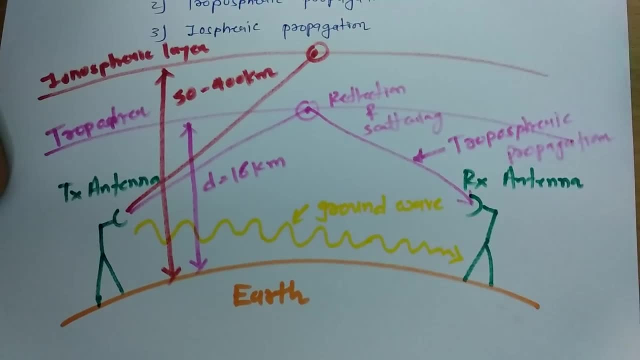 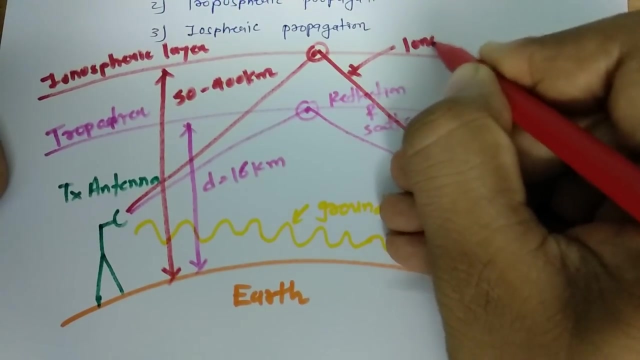 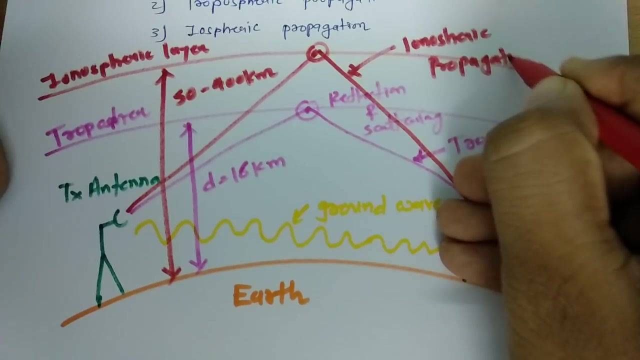 based on reflection and scattering. again it is getting reflected back on the earth's surface and it is getting received by receiving antenna. So this is what ionospheric propagation. Now, when we talk about these two propagation- tropospheric propagation and ionospheric propagation- 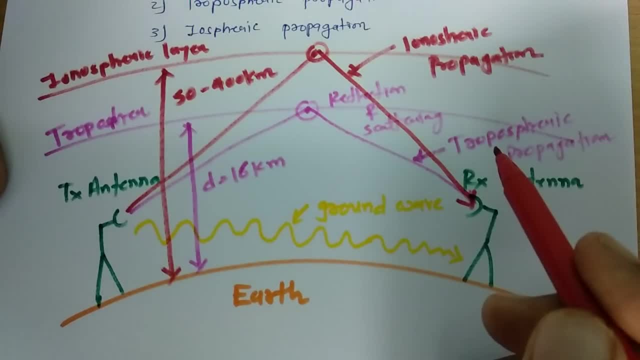 So what happens is when we send signal from transmitting antenna to ionospheric layer, it is getting Tanalar propagation. Now it is worthy to note that two microscopic propagation and senzafic propagation is also good. So all these things together is called tropospheric propagation and seed propagation. 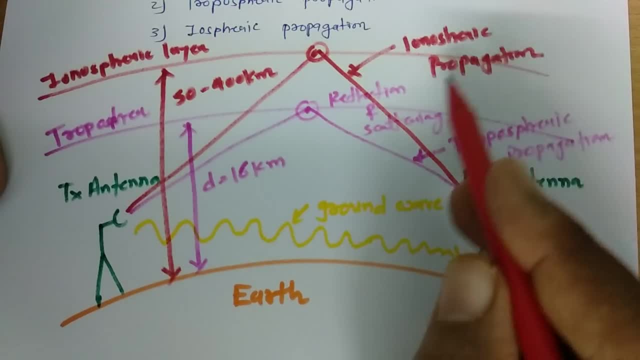 So further they are common and communicate with each other. So, similarly, compos, stereotype propagation can beaker and hydrophobic propagation are combined together, which is called sky-wave propagation. So right, we talked about these two things earlier. Now let us discuss tropospheric propagation, and in tutte more detail. 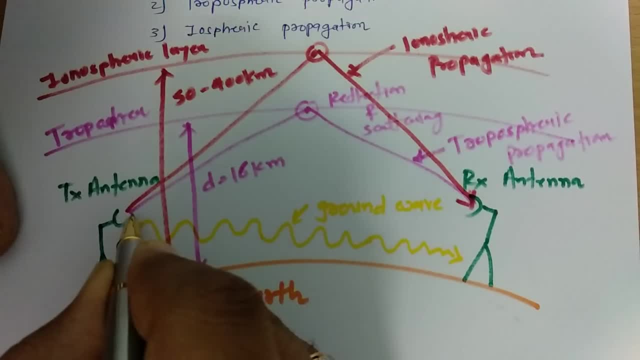 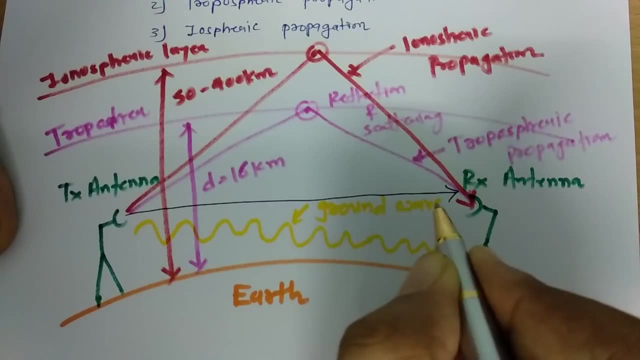 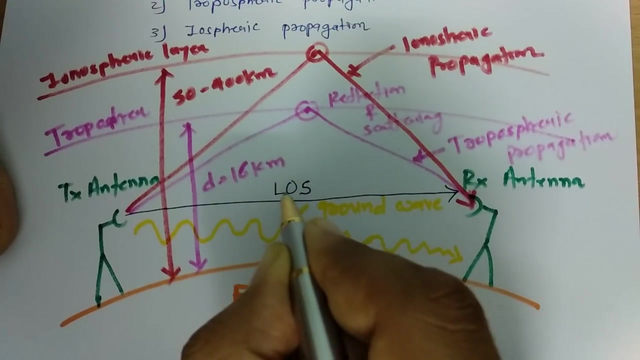 Now, if a signal starts to transfer a second, with this Aquí one step, it does not give feedback, as now 236V selected, so we are going to go double step from transmitting antenna to receiving antenna. So this is, one can say, LOS line of sight propagation. 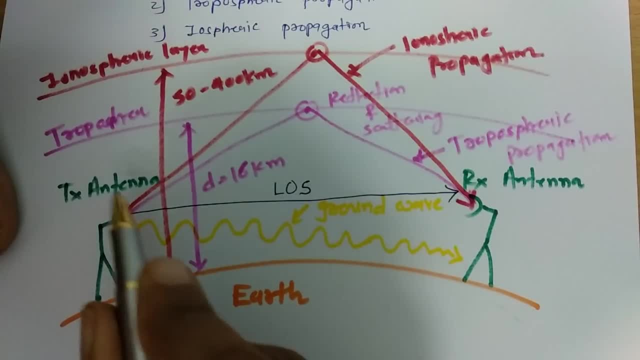 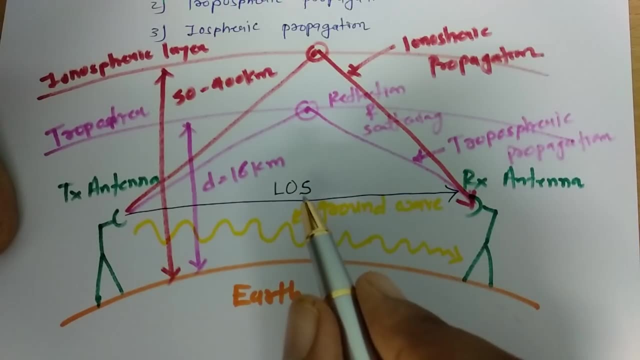 in which we send signal from transmitting antenna to receiving antenna by a straight path. So that is, what line of sight that is not propagating along with ground? In ground wave propagation signal propagates along with ground, while in case of line of sight propagation signal directly goes from transmitting antenna to receiving antenna. 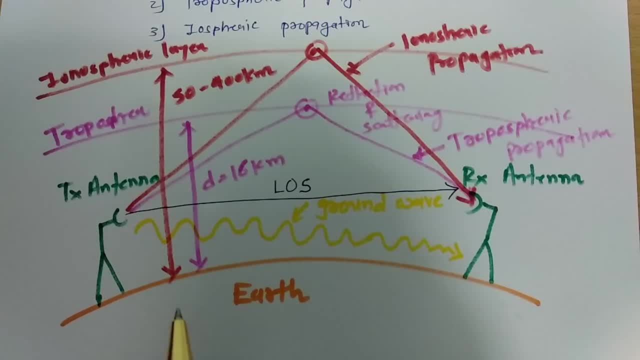 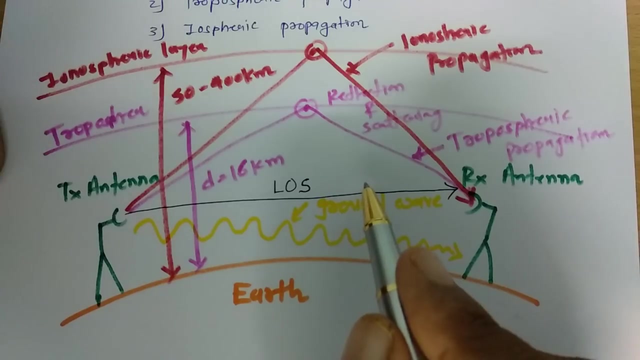 So this is what about line of sight propagation? In next few videos I will be going to explain detailed understanding of all those four propagation methods with different parameters, How it happens, where it happens, what are the things about which it should be understood that I will be going to explain. 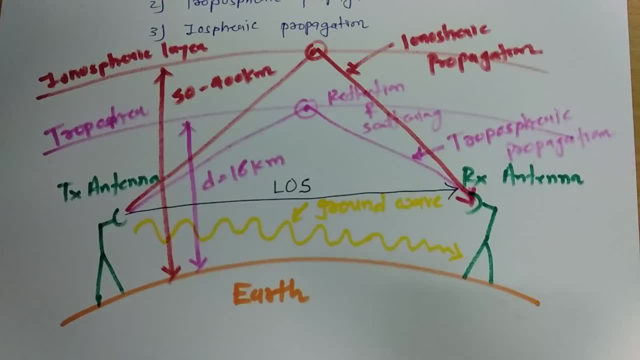 In next sessions. Thank you so much for watching this video And you can suggest me those videos which is required to complete antenna and wave propagation playlist, If I have understanding based on your need. definitely I will place videos based on your need and I will try to sort out those queries.